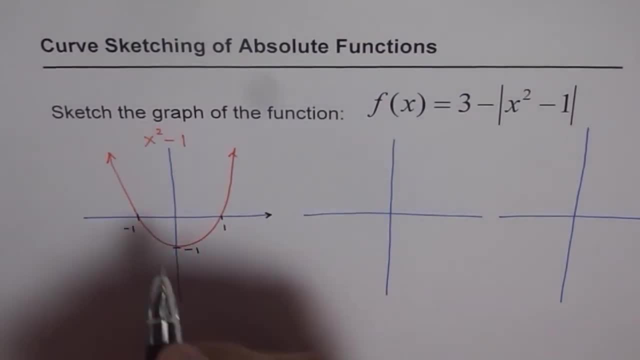 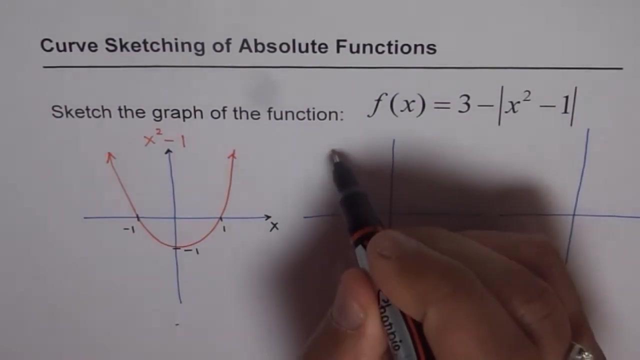 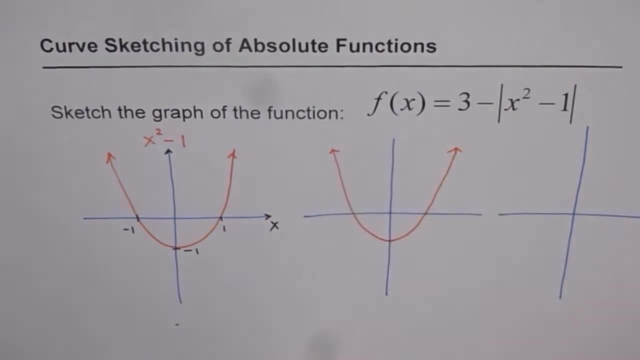 and minus 1.. And that fairly well represents x squared minus 1.. So that's what we have. So on the y-axis we have x squared minus 1.. Now, if I have to make absolute of this function, then what should I do? So what I have here is kind of my function like this: Right, So this is my x squared minus 1.. Now, if I have to do absolute of this function, then in that case, how can I? 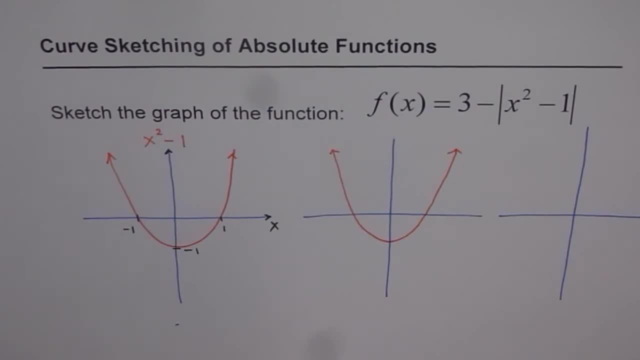 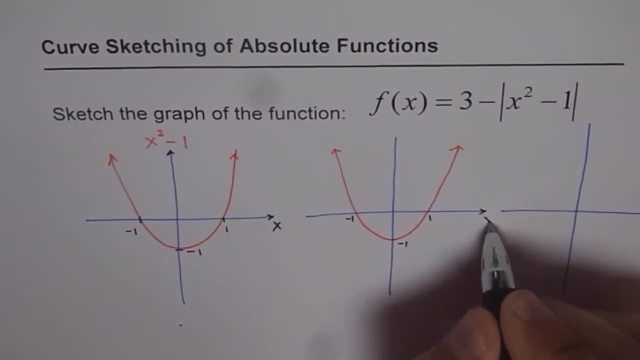 change it to absolute function. Now, as you know, we'll just copy those values, which is minus 1, minus 1 and 1.. And that is x for us. And now what we are trying to do here is make absolute function. So absolute means all positive values, So these values will kind of flip over, So we'll have the part of the curve like this now. So this graph represents: 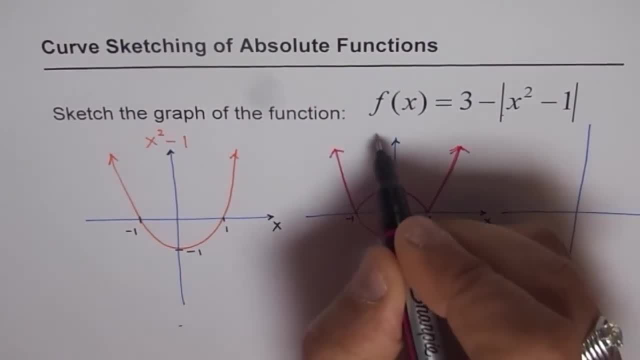 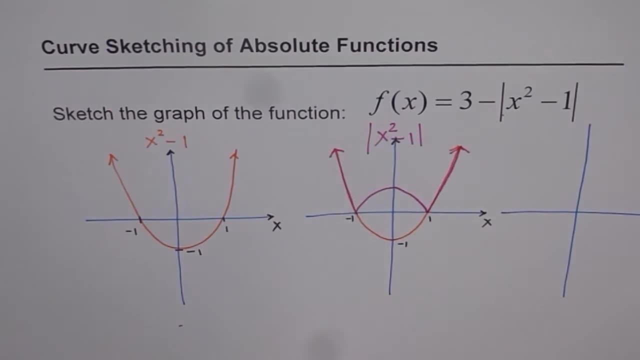 absolute value: Right Absolute of x squared minus 1.. So that is absolute of x squared minus 1.. Correct Now the next one is reflection. Right Minus indicates reflection, So we need to reflect this graph, and 3 indicates translating 3 units up. So that is the final stage where we are going to do translation and reflection. 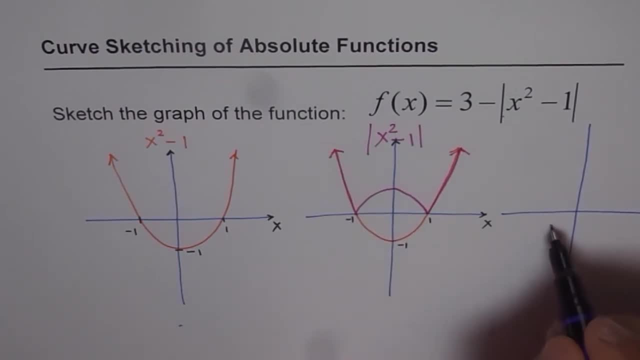 So if you reflect it, it kind of becomes like this: Right, So that is kind of reflection, and these sides will be coming down Right, That is the reflection Right Now. what we have to do is move 3 units up. So if we move 3 units up, it's kind of coming at this point. Is that okay? So what are we going to get? So these points, all the points, will move 3 units up, So we'll get points here and that one will come kind of here. Do you see that? 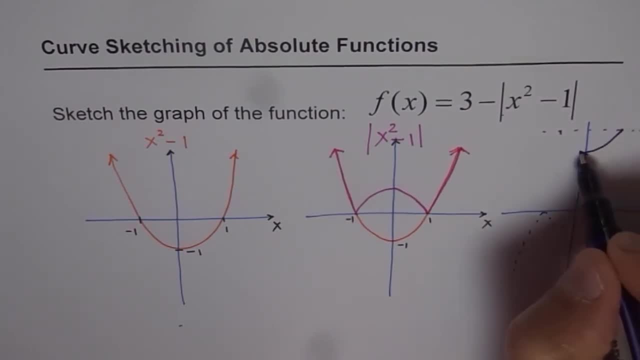 So our graph will look like something like this: Do you see that? Now let me just move it down and we can always find what are the zeros later, Right, But anyway. so we got our function, but these are the 3 steps in which we could do our final graph, and that is the function f of x. Do you see that? Now, of course, to find the x squared, 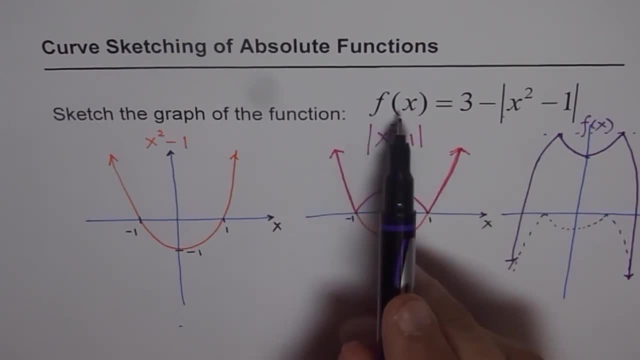 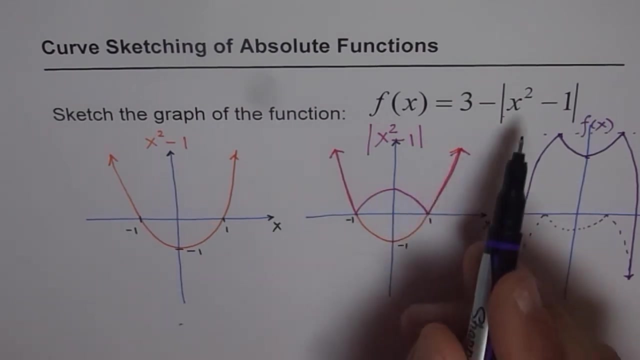 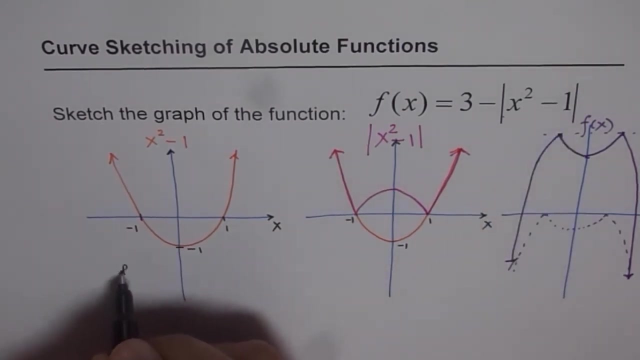 intercepts. what you can do is you can substitute the value of f of x as 0 and then figure it out, Right? So that's one way we can do it, Anyway. so let's recap the steps. So in step 1, plot x squared minus 1.. That is the first step. And then you do absolute it, Right? So first you plot x squared minus 1.. That is step 1.. 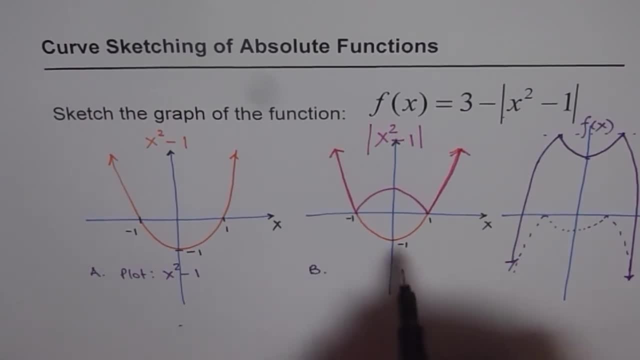 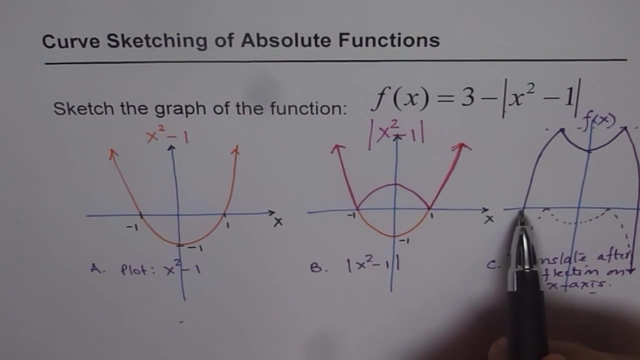 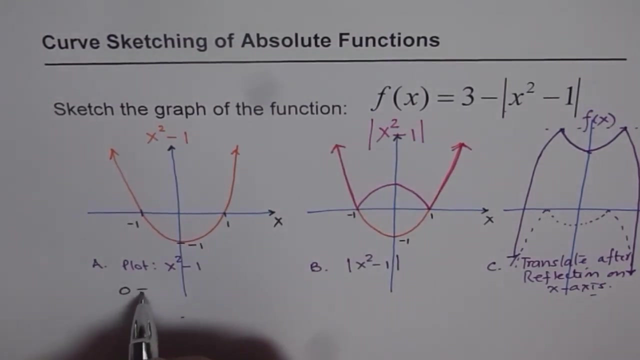 Step A and step B is you do absolute of x squared minus 1, and that is to say that you make all negatives as positives and keep positive as such. Right, That's what it means. And the last stage is translate, after reflection On x axis, Right To get the final graph Right. So, as an exercise, what we should also do is to figure out what are the x intercepts in this particular case. Right, That means when f of x equals to 0. So we can calculate this: We get 0 equals to 3 minus x squared minus 1.. So x squared minus 1: absolute, as you can see. 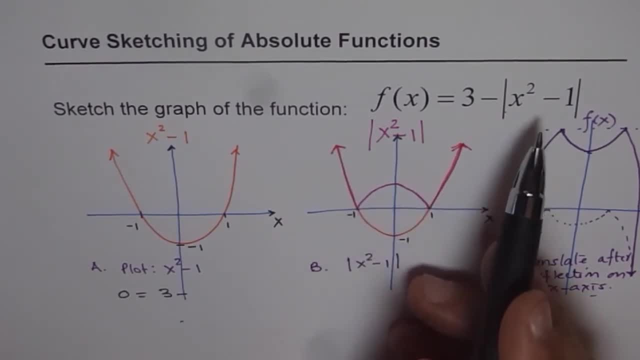 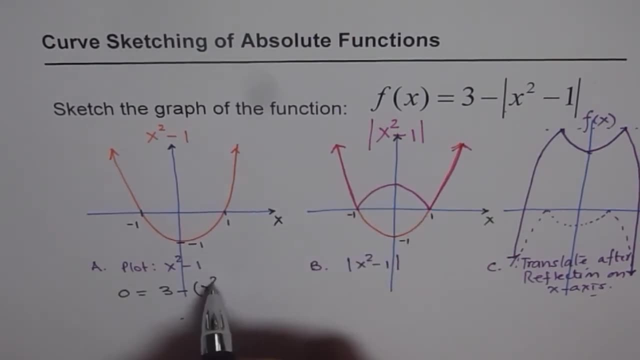 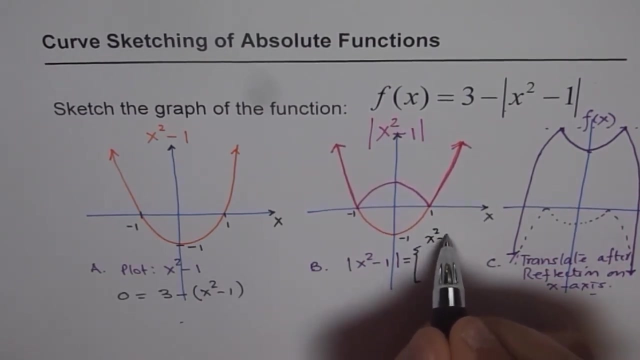 Is x squared minus 1.. If you are going beyond plus and minus 1.. Right, So we should say we can use here the value x squared minus 1 itself. Right, Since the function is defined that way, you can see here that the absolute function is actually equals to- let me define it here- is equals to x squared minus 1.. If, If absolute value of x.